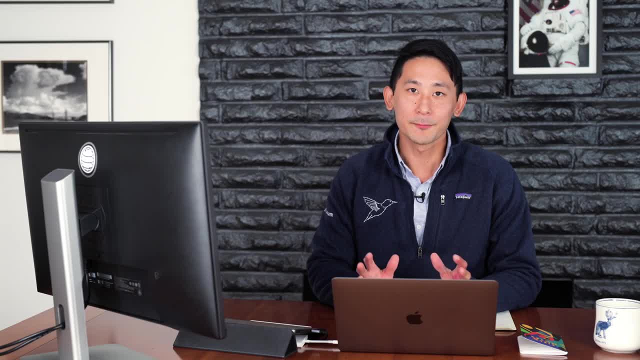 thousand years of processing time on a typical laptop. Quantum computers running Shor's algorithm could one day shorten this wait significantly, but quantum processors today are far from being able to do this, So you don't need to worry about your credit card transactions anytime soon. 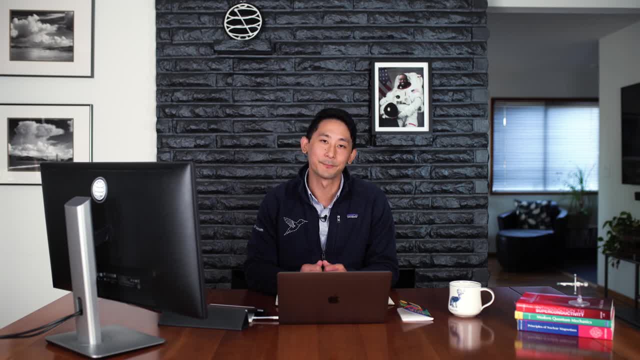 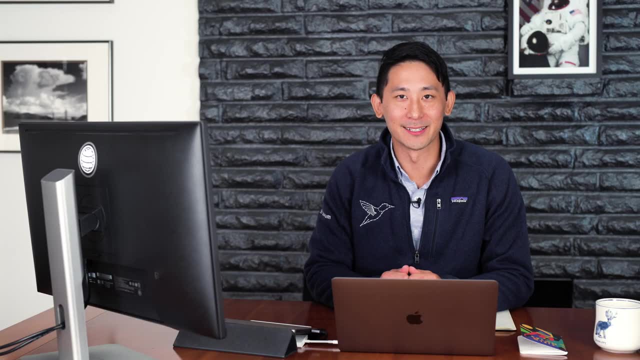 In this episode we'll focus on how to implement Shor's algorithm in Qiskit, but if you want to learn more about the theory of Shor's algorithm, check out the links in the description below. So let's actually implement Shor's algorithm now in Qiskit. 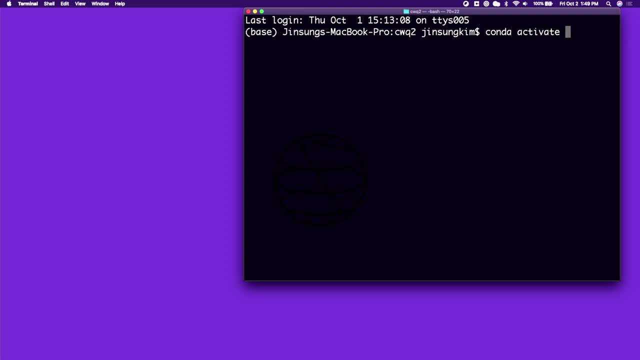 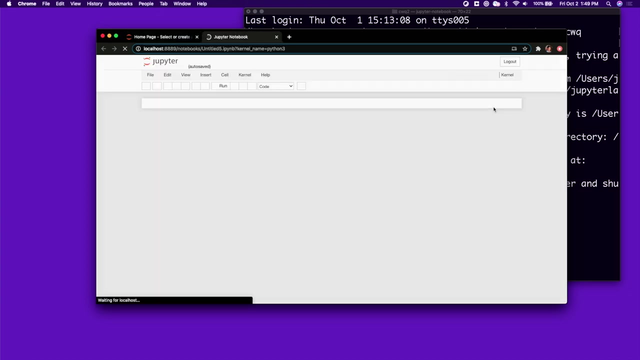 All right. so first, as always, I'm going to activate my Qiskit environment. going with Qiskit, This is where I have Qiskit installed- I'm going to open up a Jupyter notebook, Open up a new Python 3 notebook. All right, so the easiest way to run Shor's algorithm is to use 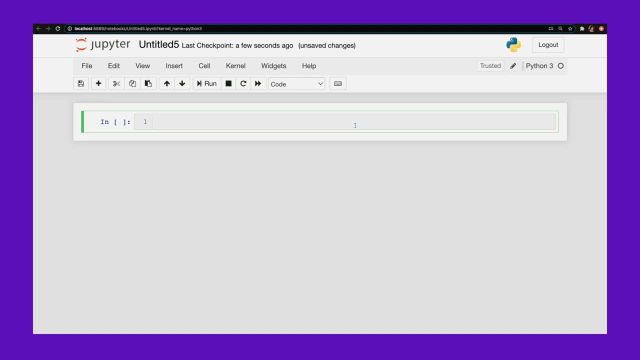 the Shor class in Aqua. So from Qiskit Aqua algorithms I'm going to import Shor. I'm going to also import quantum instance from Aqua and this is going to run my experiment: Import NumPy. Let's see if this works. 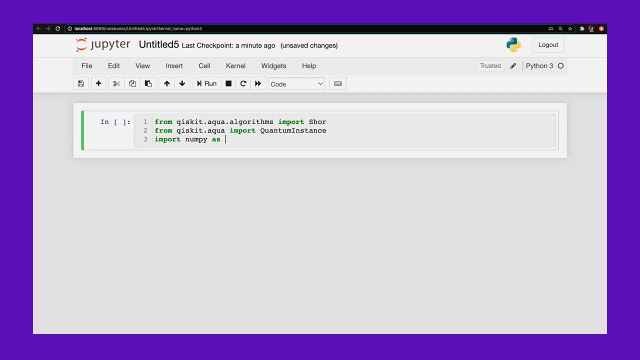 All right, let's see if this works. And let me also import quantum circuit air and execute. These are all the things that will run my experiment And from Qiskit tools visualization, import plot histogram so I can look at my results. 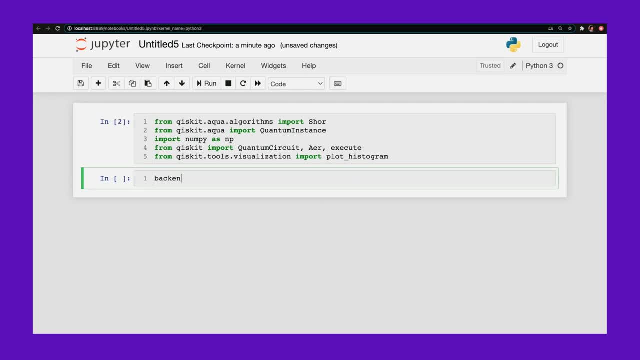 Oops, Import. Okay, so let me set my back end to the Chasm simulator. I'm going to set up my quantum instance to run my experiment. Plug in my back end, Say shots is 1000.. Well, that's set my Shor's algorithm. 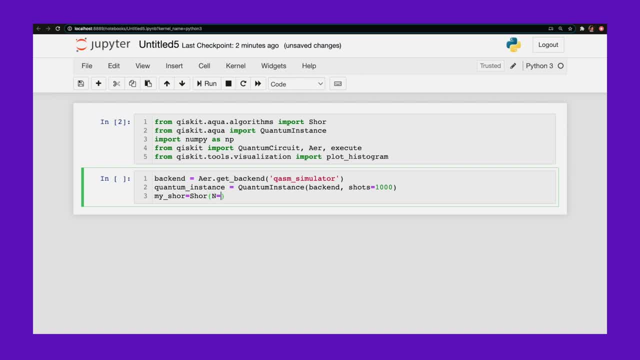 And so for this example, I'm going to factorize the number 15.. N is equal to 15.. This is just a really simple example, just to show you what's going on. I'm going to talk about what this A number is in a little bit, All right. 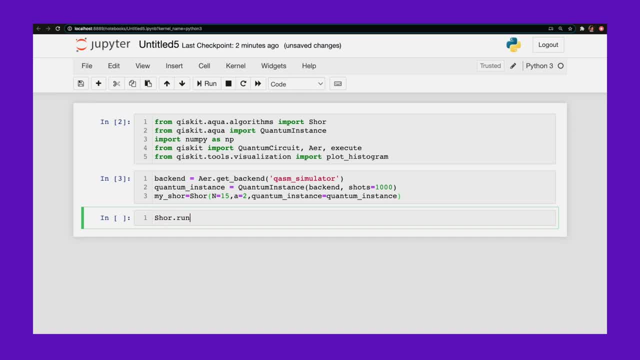 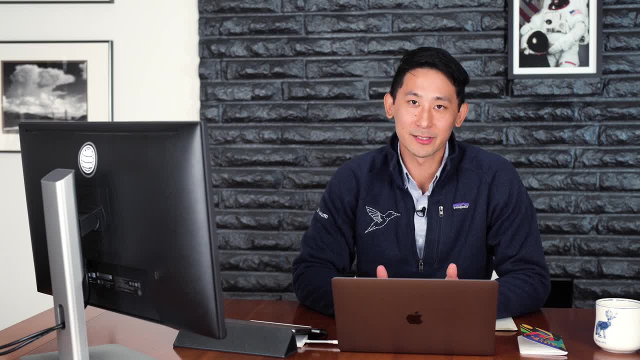 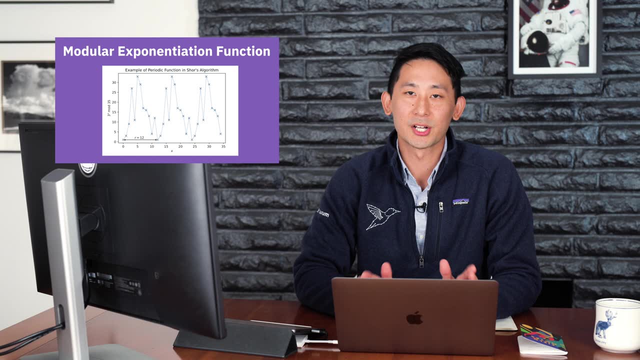 Let's take a look at how the algorithm is actually built. Shor's algorithm can be broken up into three parts. Number one: we can convert the factoring problem into a period finding problem using what's called the modular exponentiation function. What this boils down to is 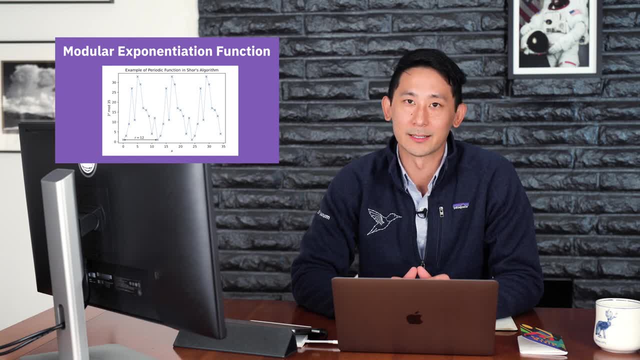 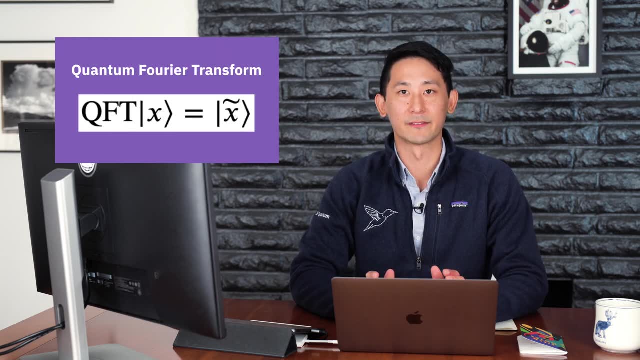 dividing our number by a guess number A, and computing the remainder For good guesses of A. this function is periodic as we increase the power of A. The second part finds the period of the modular exponentiation function using the quantum Fourier transform, And this is: 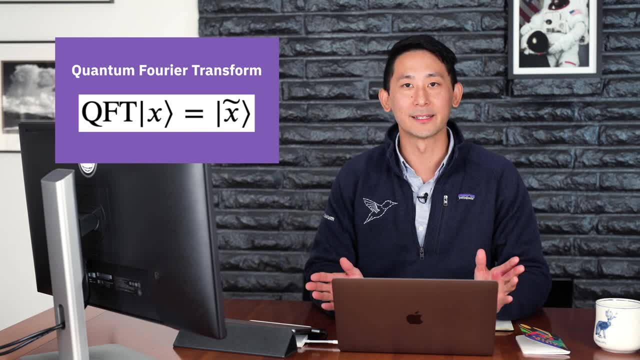 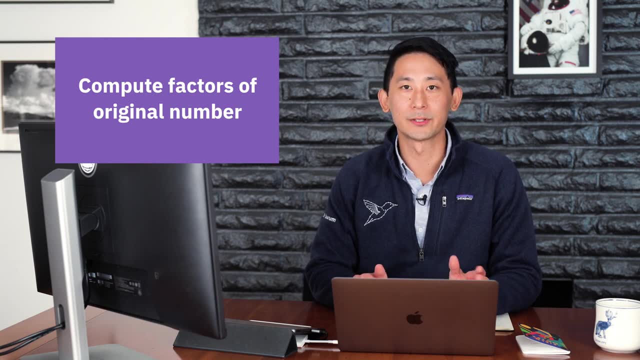 responsible for the quantum speedup of this algorithm. And finally, number three: once we found the period of our modular exponentiation function, we can use this number to efficiently compute the factors of our original number using the following magic formula: So we're going to 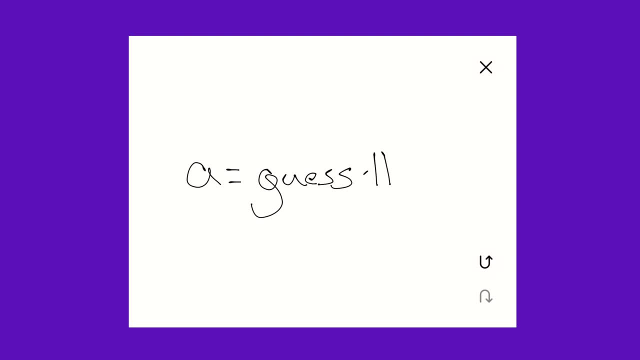 take our guess, number A, and we're going to take the period of our modular exponentiation function, And these are our two magic numbers: P is equal to A to the R over two minus one, And Q is equal to A to the R over two plus one, And N is our. 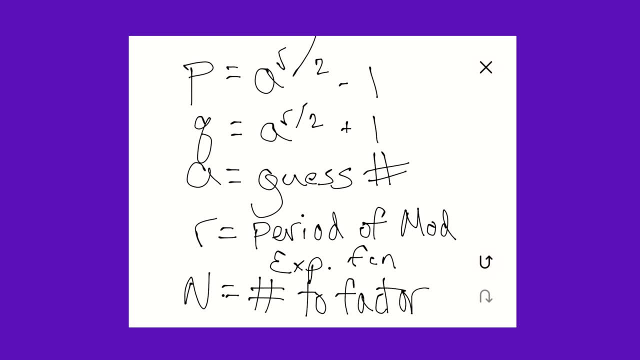 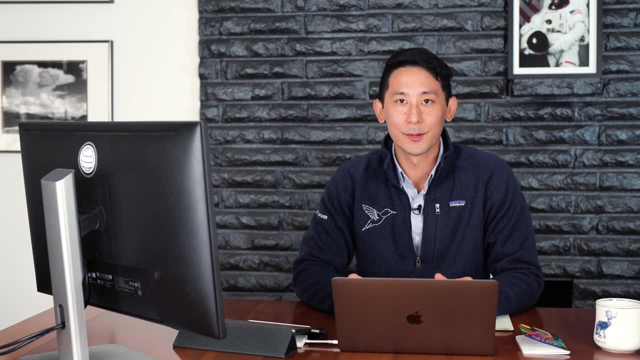 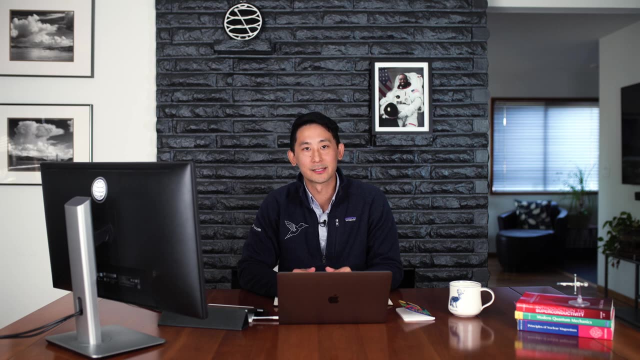 number that we're trying to factor. So these two magic numbers, P and Q, are not necessarily the factors of N that we're looking for, But with high probability they'll have cofactors with N which we can compute efficiently. And if our magic numbers aren't integers, we can just use another guess for A. 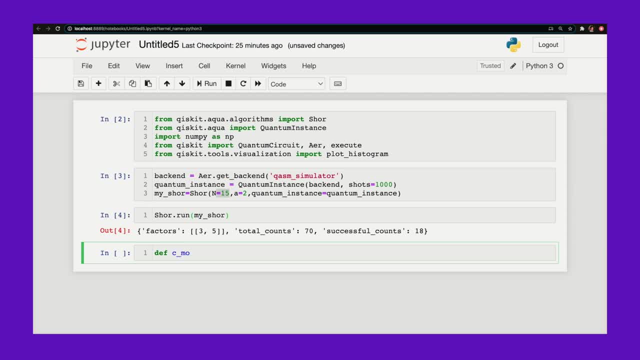 So the first thing I'm going to do is code up my modular exponentiation function, And this is hard coded for factorizing 15, and also hard coded for a guess number of seven. Generally, you can construct circuits efficiently for whatever guess you're trying to use. 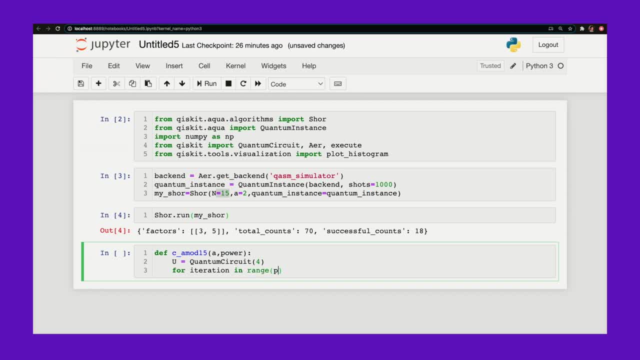 For iteration in range power, And all this circuit involves is doing a few swaps: One, two, You swap zero, one, And then for Q in range four, do an X gate. Okay, I'm going to turn this circuit into a. 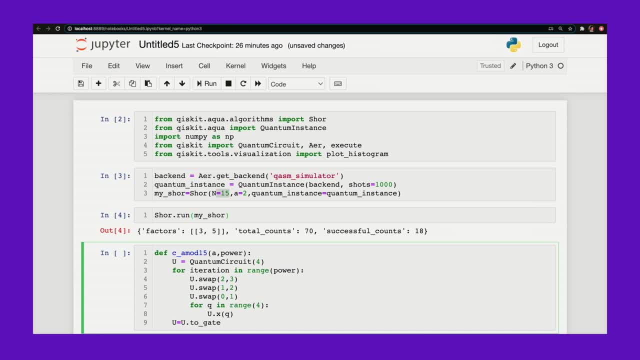 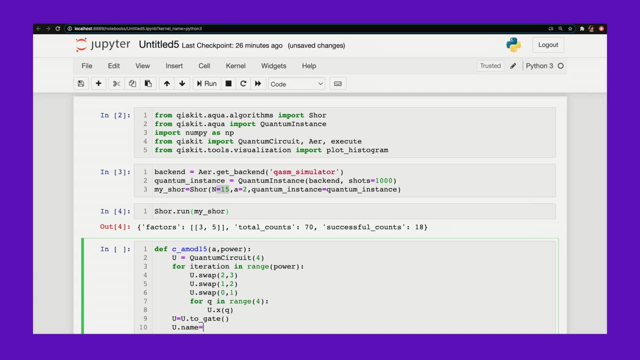 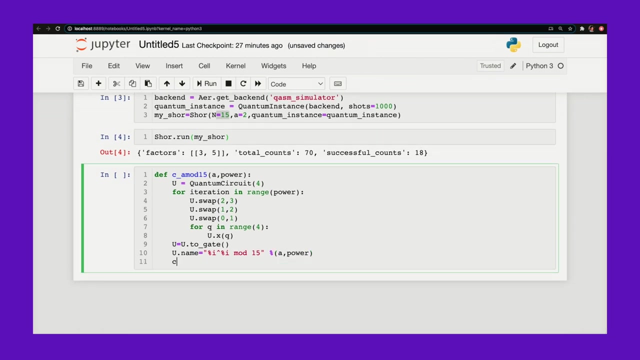 gate so we can plug it in to our Shor's algorithm later. Let me just name this circuit equal to mod 15.. And 15 is once again the number that we're going to be factorizing in power. Okay, out of control. 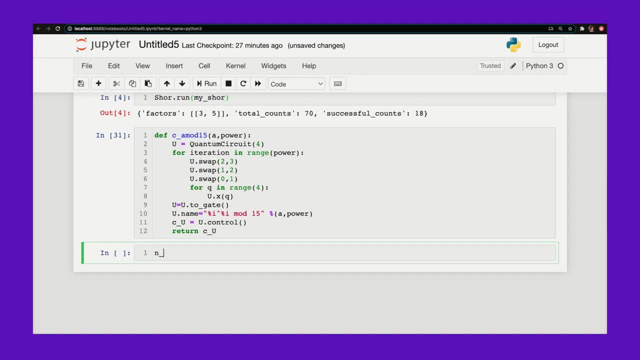 Okay, So we're going to specify that we have eight qubits that are going to be counting our exponent And our guess number A is going to be seven. All right, so now I'm going to define my quantum Fourier transform circuit. So my quantum circuit will take: 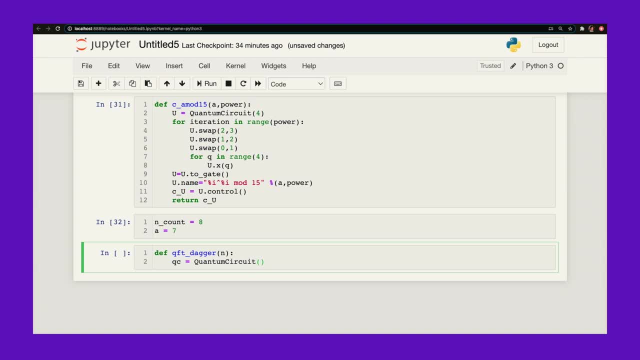 n qubits for qubit range: n QC. swap these qubits around: n minus qubit minus one, and then I'm going to take the other qubit and I'm going to take the other qubit and I'm going to take the other qubit. 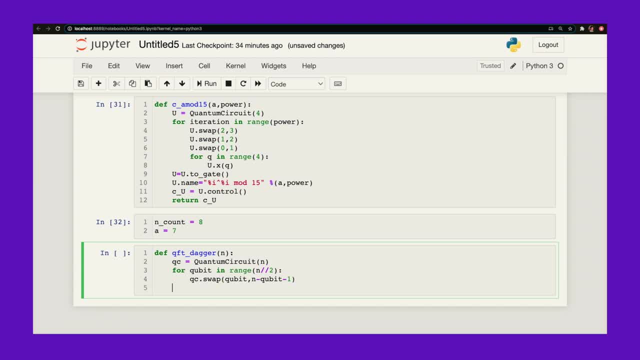 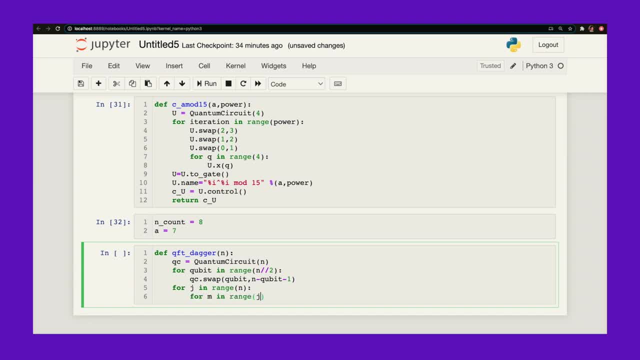 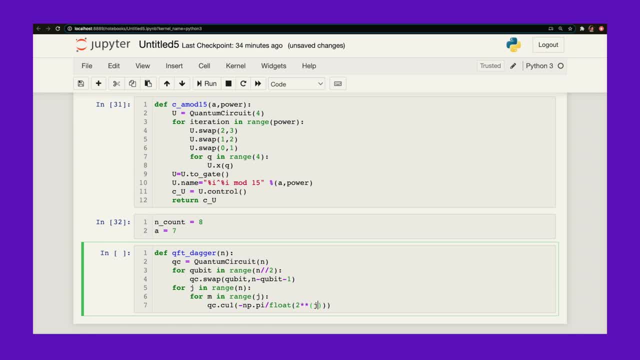 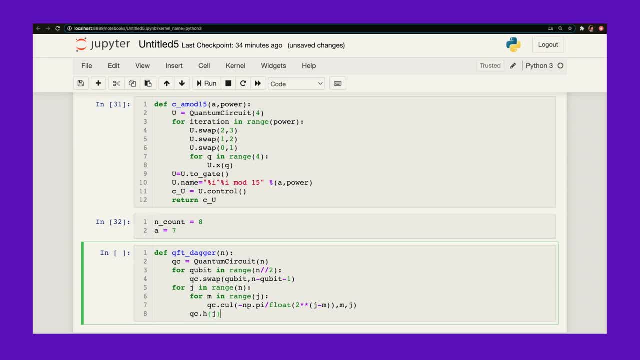 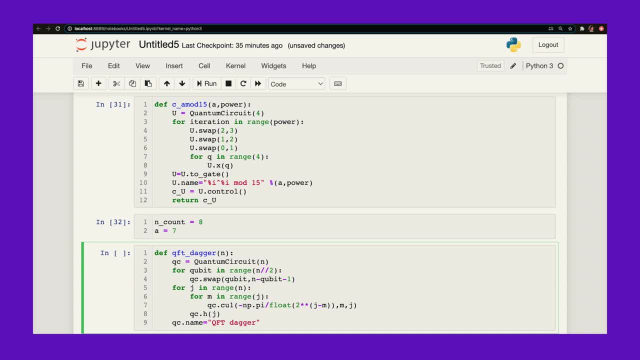 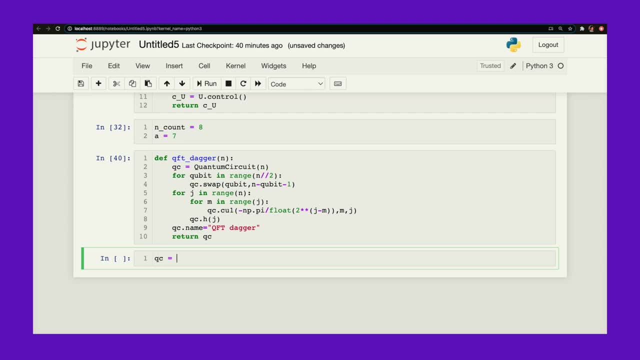 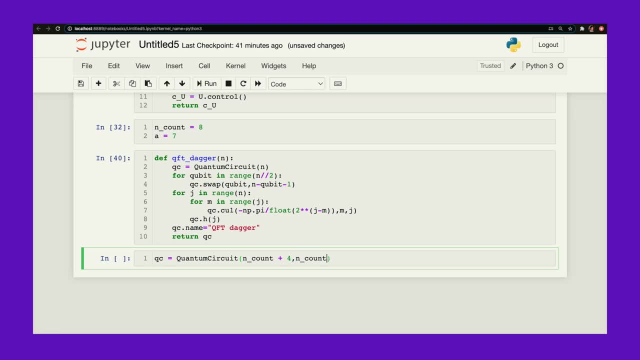 and then I'm going to take the other qubit. I'm going to initialize my counting qubits into a superposition state. Just do some Hadamards on each qubit. I'm going to initialize my first ancilla in the excited state. I'm just going to flip. 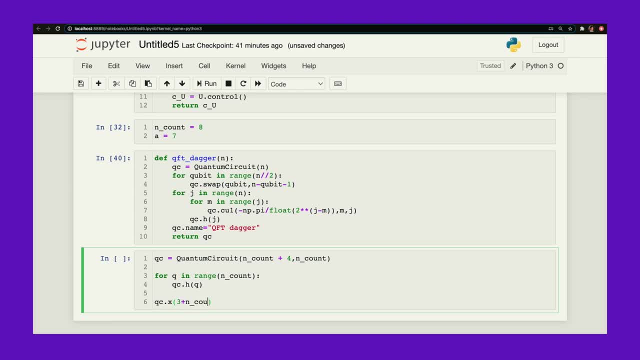 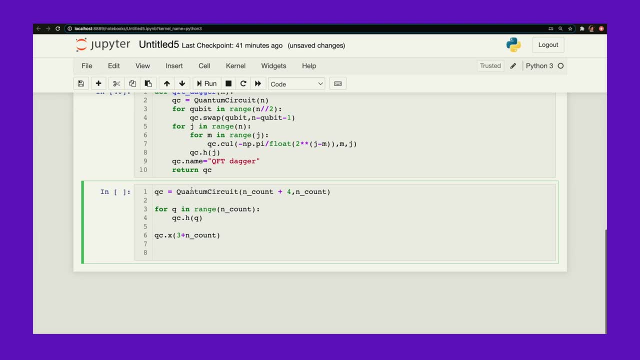 it with an x- x gate. all right, so now let's add my modular exponentiation function. append. this is my modular exponentiation function. Okay, And this is hard-coded, for a is equal to seven and there's other circuits for other guesses. 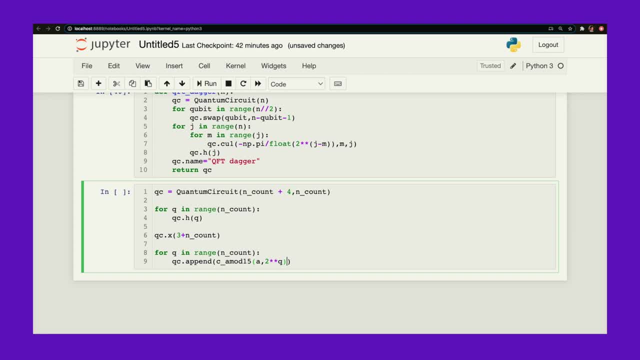 of a Q plus i plus n, count for i in range four. okay, and I'm going to do my quantum Fourier transform. Okay, And finally, I'm going to measure my circuit. Okay, let's see what this looks like. 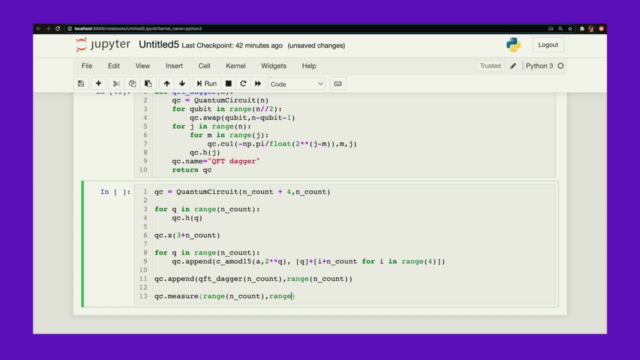 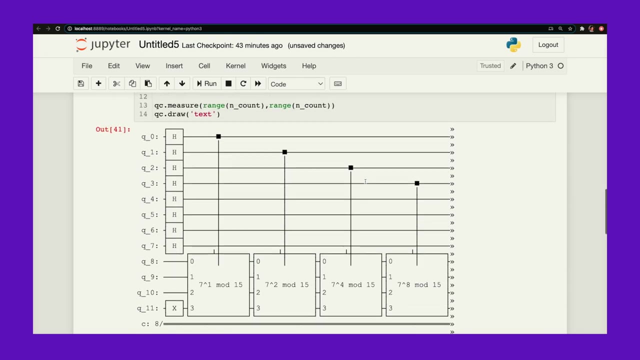 Okay, I'm going to do my quantum Fourier transform. Okay, I'm going to do my quantum Fourier transform. Okay, I'm going to do my quantum Fourier transform, Okay, All right. good, So I've initialized my counting qubits into the superposition state. I'm applying my modular 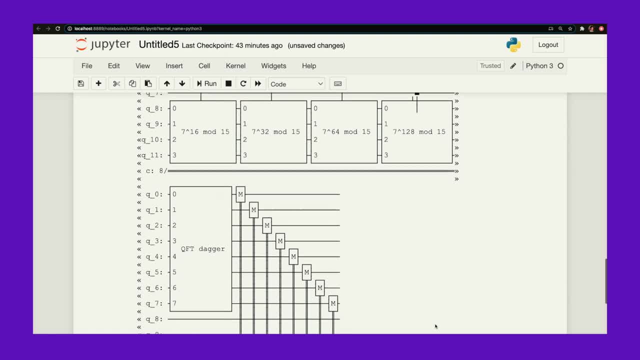 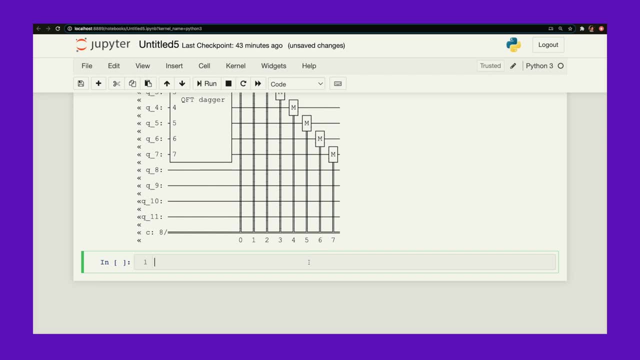 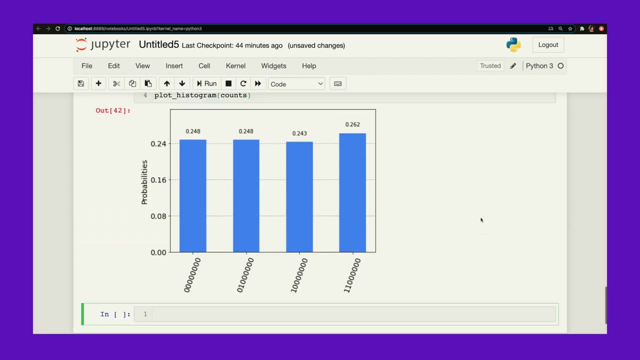 exponentiation function, and then I do my quantum Fourier, transform at the end and measure. So now let's actually execute this on one of the simulators. I'm going to use the chasm simulator. Okay, I'm going to look at the formula. I'm going to use the expectation function and I'm going 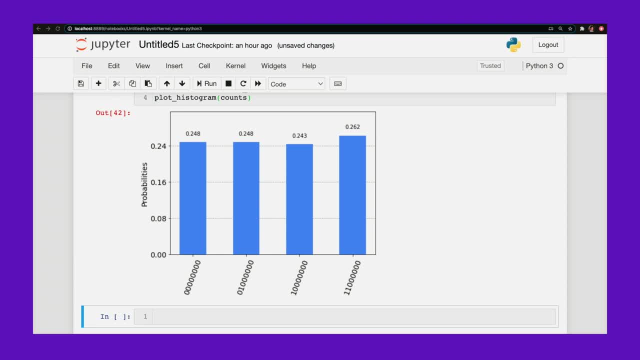 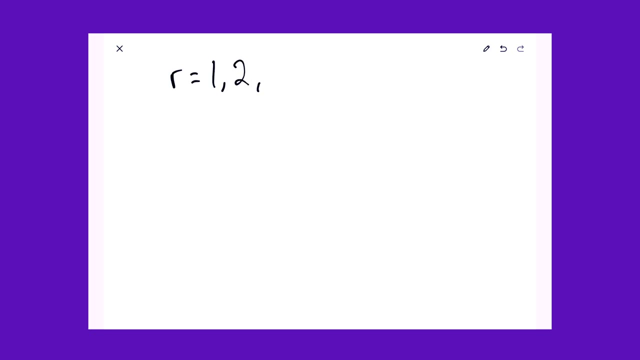 to. So let's look at the value r is equal to 4 and plug it into our magic formula, which is: p is equal to a to the r over 2 minus 1, and q is equal to a to the r over 2 plus 1.. 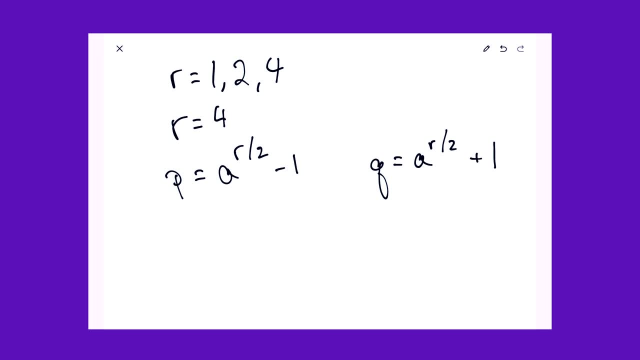 And remember that p and q are not necessarily the factors. of our original n is equal to 15, but I claim that they have cofactors with n which we can find efficiently. So if we plug r into our formulas, p is equal to 7 squared minus 1, a, remember, is equal to 7..